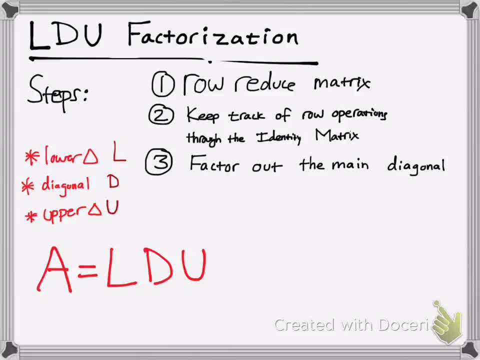 And how I like to think about it is similar to L-U decomposition. it's very similar. How I like to think about it is: well, A is your matrix right, And it can be split up into three different parts, in this case. 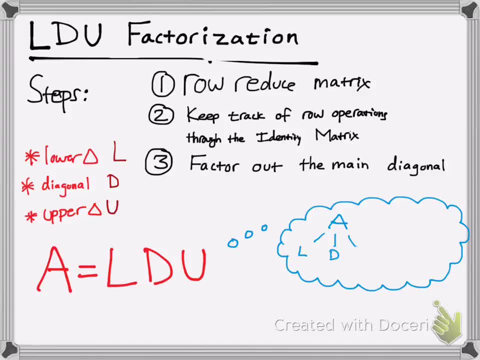 So you have your lower triangular matrix, your diagonal matrix, your main diagonal and your upper triangular matrix. Now this can be similar to like taking factorization. You have 12.. What else can 12 be written as? 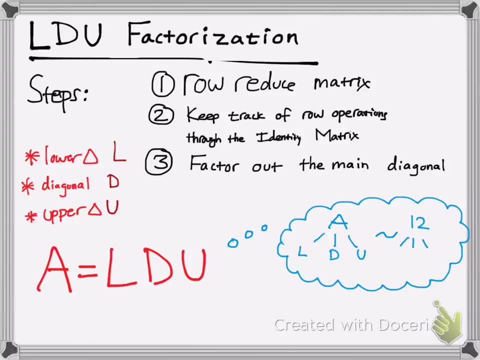 Well, it can be written in three different numbers. when you factor it down right, 3 times 2 times 2, to make up 12.. So it's kind of like the same thing we're doing. it's very comparable. 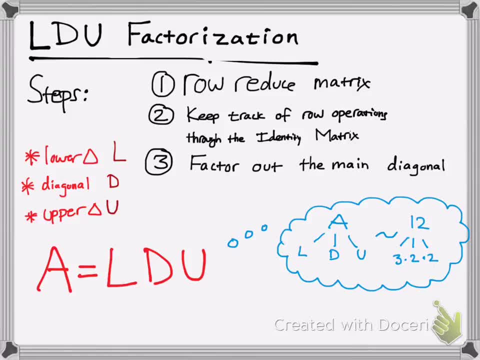 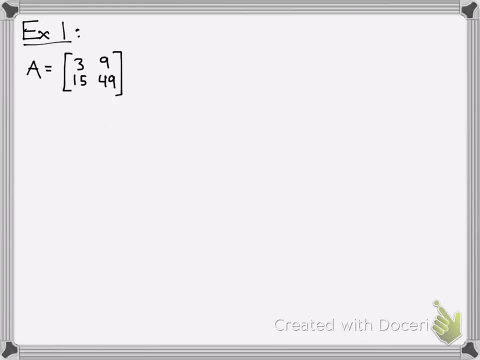 It's kind of like an analogy of what we're doing for L-D-U factorization. So let's take this example. We'll do this. one first Example, one first. So we got a 2x2 matrix. I'd encourage you to pause the video and do simple row reduction. 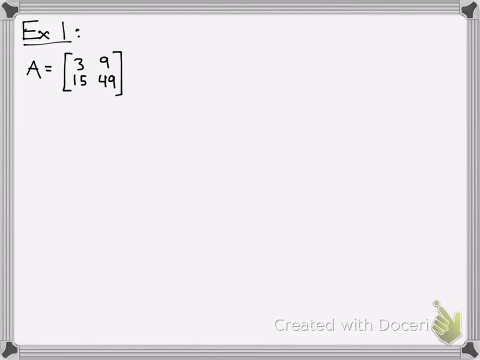 I'm going to go through this. I'm going to do this fairly quickly in terms of the row reduction steps. So you have 3, 9,, 15,, 49.. You want to make your pivot is 3.. 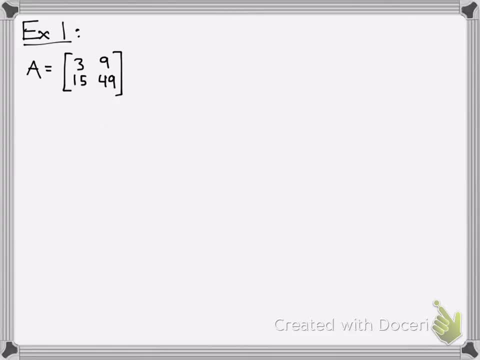 And you want to get rid of the 15 and make it a 0 on the bottom. So what you do? you add negative 5 times row 1 to row 2. And you should get 3,, 9,, 0, 4.. 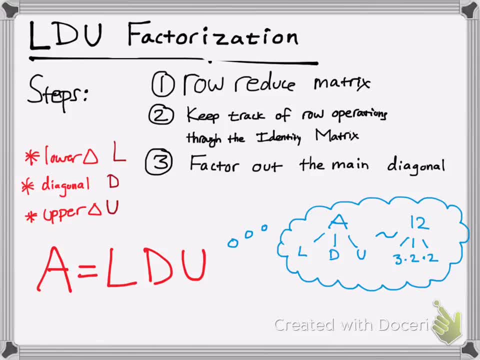 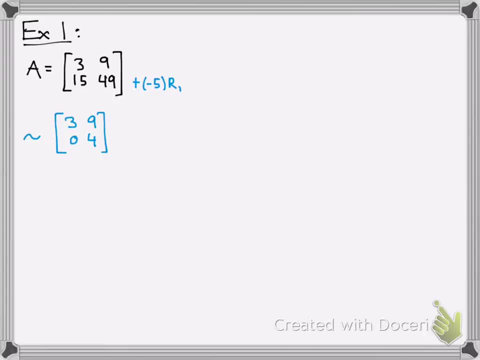 Now pretty easy. What do we do next? Well, we have to factor out the main diagonal. So I'm kind of going a little out of order here, because we'll have to keep track of our steps later. But I'd suggest factoring out the main diagonal. 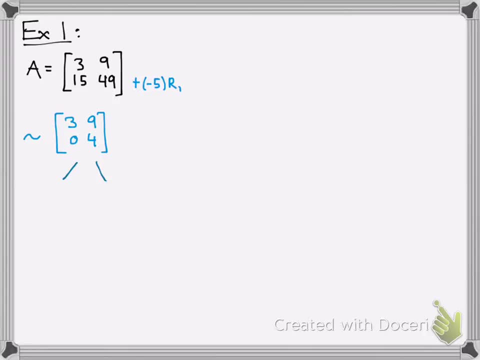 So the main diagonal is what? 3 and 4, right, So all you do is write the main diagonal and pull the numbers out, and the rest are 0.. Okay, Now, when you pull out those numbers, you're also dividing by 3 in the first row, for example: 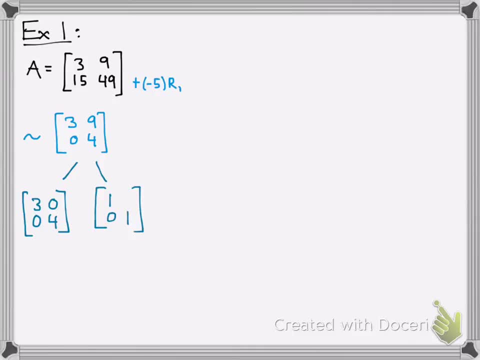 So when you divide 3 out like that, you should get 1 in the main diagonal. When you divide out 4 in the second one, you should get 1 on the main diagonal of the second matrix here. And when you take 9 divided by 3,. 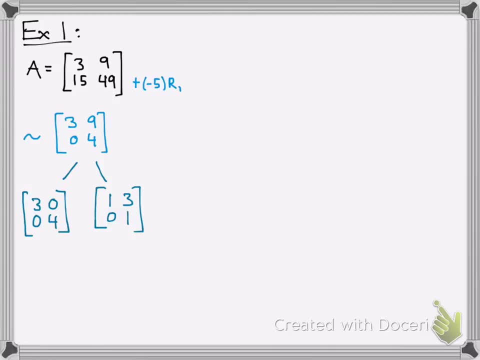 you should get 3 when you factor out that 3 there. So you have your D, you have your U. Now let's go find our L. So we have to keep track of what we did. So we subtracted 5 times. 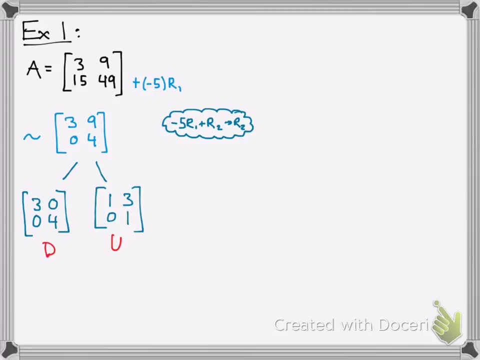 or we multiplied negative 5 times row 1 plus row 2 to yield our new row 2 when we were reduced. So you're going to do the opposite on the identity matrix. So you start with your identity matrix and you're going to perform the opposite operations. 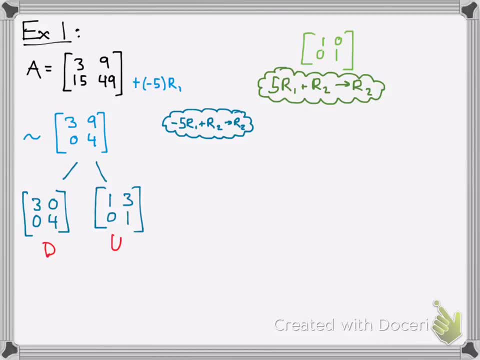 instead of multiplying by negative- So negative 5 times row 1, you're going to multiply by positive 5 times row 1 plus row 2.. So what would that look like? That's an elementary matrix, And remember, elementary matrices are the action done onto the matrix. 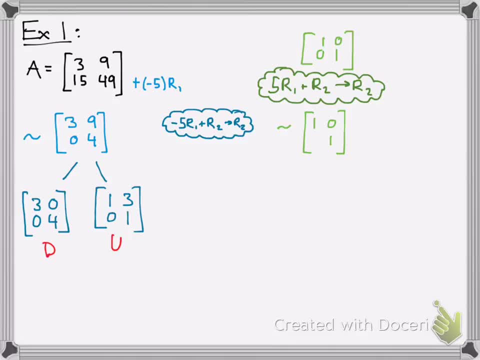 That's what it represents, the action. So we're going in the first row, right, We're multiplying 5 times row 1 to row 2.. So the action is done on row 2.. So we're going to the second row. 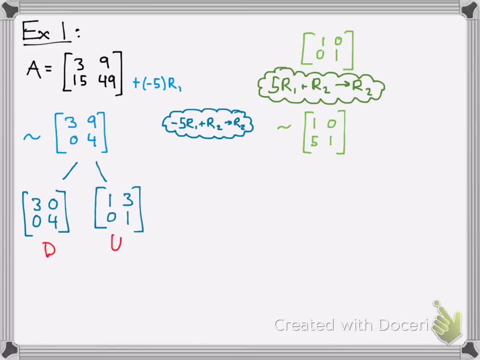 and we're doing it from row 1.. So you put the 5 there in the bottom left. Again, review your elementary matrices if that troubles you, but that should be a fairly easy step. Cool, Then you have your lower triangular matrix. 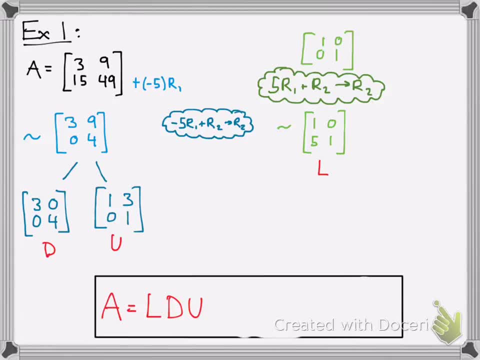 Now, well, what's the formula? A equals L D U And you just plug in what you got. You just put all the pieces together: L D U. Cool, That's L D U factorization. 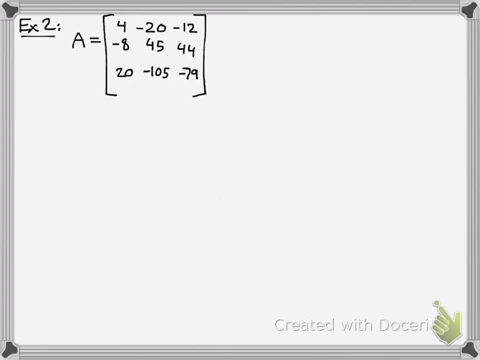 And let's do another example. Now we have a 3 by 3 matrix, So row reduction. I'm going to go through this fairly quickly. I encourage you to pause the video and see if you can do it on your own. 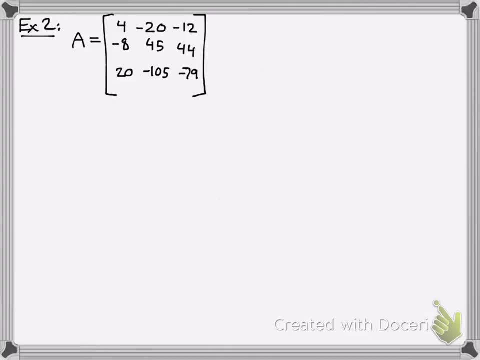 Make sure you pause it. Okay, Here we go. So 2 times row 1, negative 5 times row 1 to row 3.. You should get 4, negative 20, negative 12, 0, 5, 20, 0, negative 5, 19.. 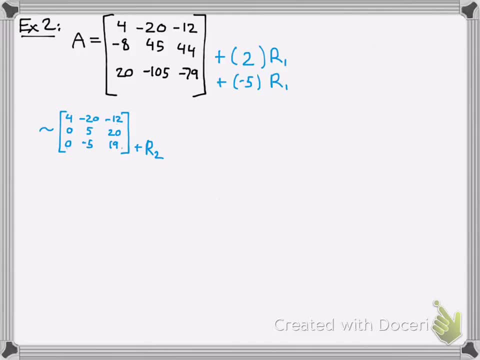 Again, you're going to want to make sure everything below the pivot is 0 to get your upper triangular matrix, And you should get this matrix here. Now that we have our upper triangular matrix, you're going to want to pull out the main diagonal. 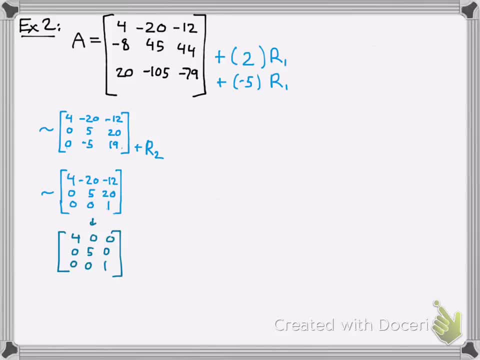 So that would be the 4,, 5, and 1. And the rest would be 0s, So you pull those out. Then, when you factor those out, that's going to also manipulate the numbers in the matrix in each row that you pulled from.